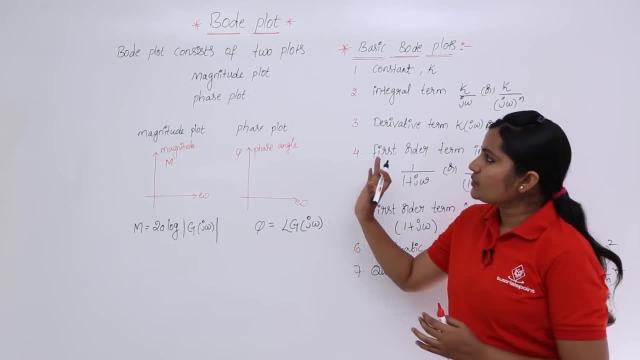 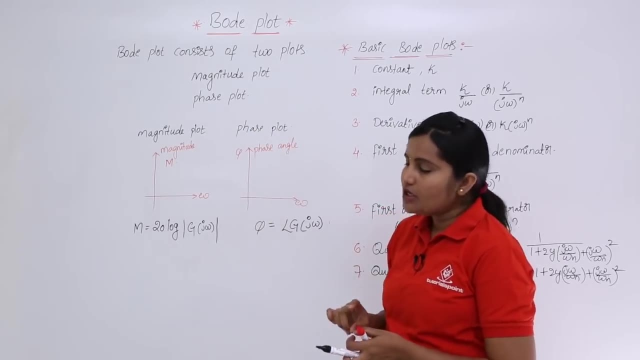 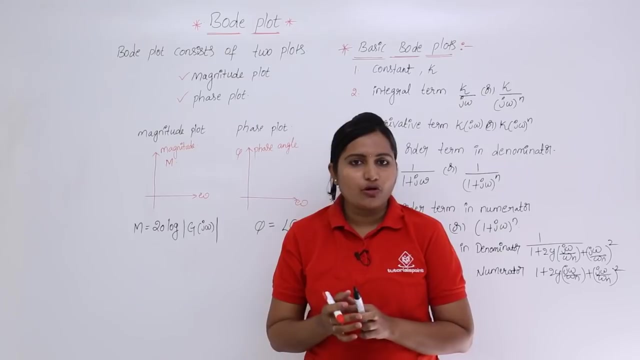 this plot in this video we are going to discuss. So here, Bode plot consists of two subplots. that plots are magnitude plot and phase plot. So these two are two subplots of Bode plot. By combining magnitude plot and phase plot we are going to get the Bode plot. So now coming to 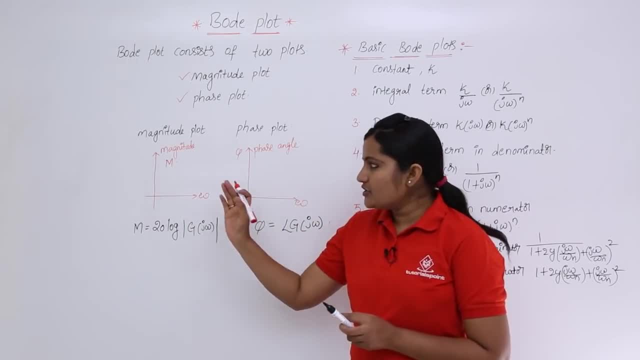 magnitude plot and phase plot. both this magnitude plot and phase plot contains the similar x axis. that means the x axis is the angular frequency, where angular frequency is equivalent to omega. So if you observe these two, these two plots, these two plots containing similar x axis, that similar x axis will be omega. that means: 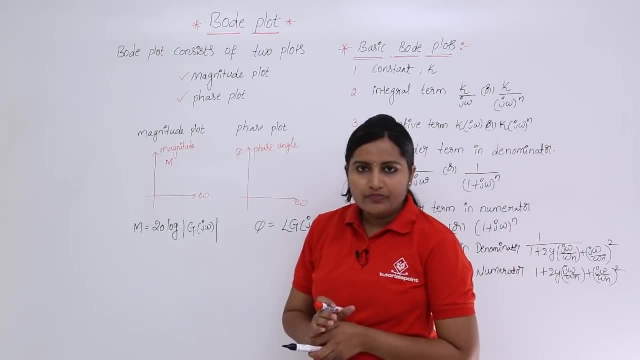 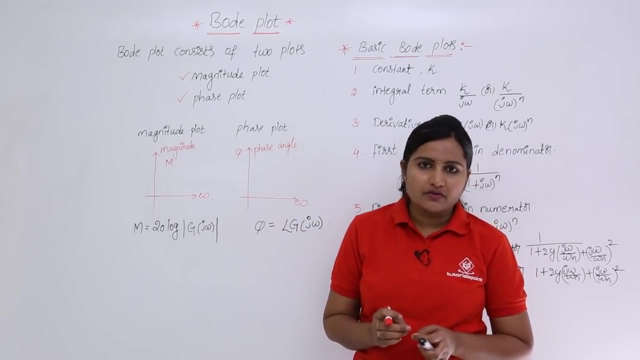 angular frequency Coming to magnitude plot, and these two plots are differ in y axis. for magnitude plot, the y axis is the magnitude of the open loop transfer function. We know how to calculate magnitude of open loop transfer function If you know open loop transfer function. 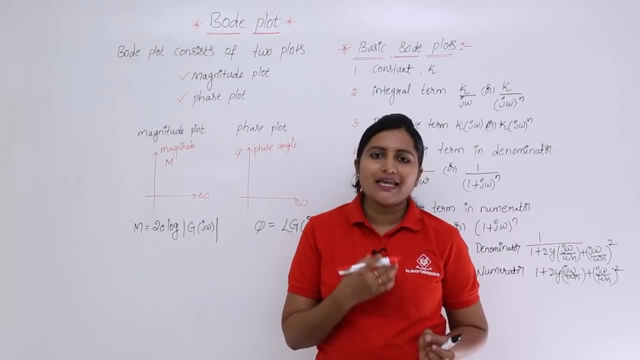 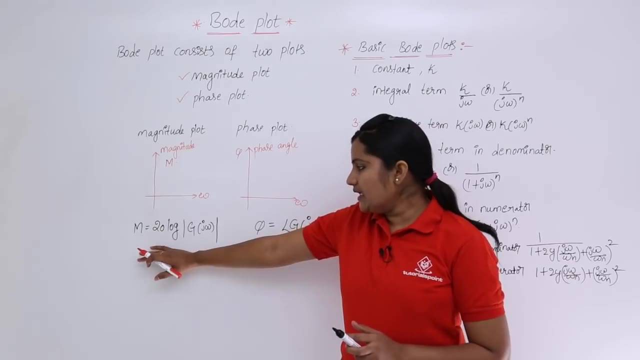 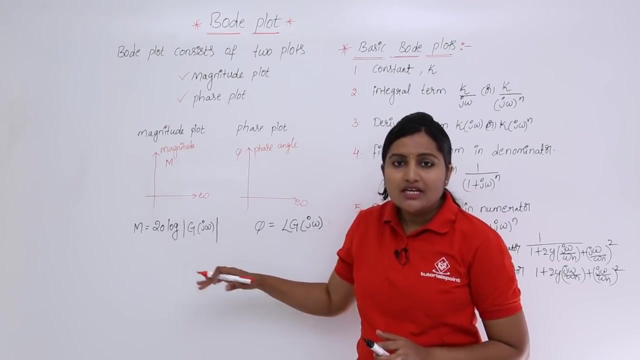 the magnitude of that open loop transfer function can be obtained by taking modulus and 20 log. So this is the magnitude: 20 log modulus of g, of j, omega will be magnitude of open loop transfer function. Generally in some textbooks you can find like this magnitude is equivalent to 20 log modulus of 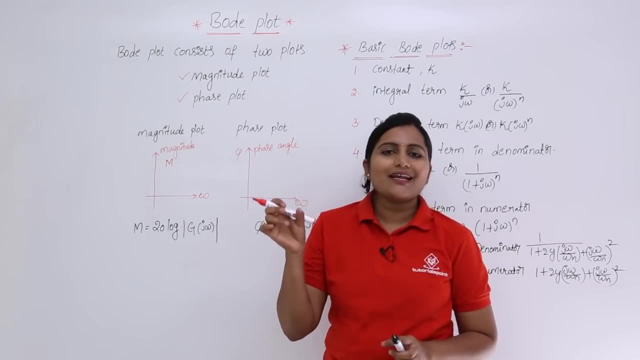 g of j omega into h of j omega, also where h of j omega is equivalent to 1.. So we are calculating all this for unity feedback system. So for unity feedback system, as h of j omega is equivalent to 1, we are not going to consider. 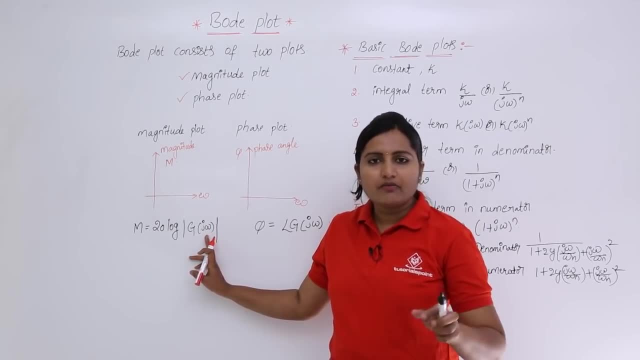 that 1.. Otherwise you can take like that also, and after one more step. you need to consider: h of j omega is equivalent to 1, and finally you need to get the same Magnitude is equivalent to 20 log modulus of g of j omega into h of j omega, where h of j omega is equivalent to 1.. So we ini. 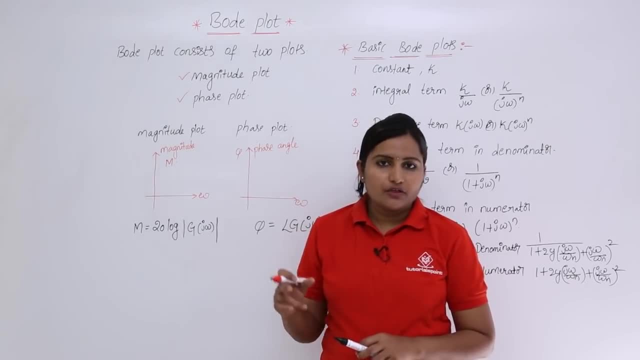 e row using all these attributes- we do might consider all these there Now, just to accurately- is equivalent to 1 for unity feedback control system. Now, finally, the magnitude, which is nothing but y axis of our magnitude plot, is equivalent to 20 log modulus of g of j omega. this omega we need. 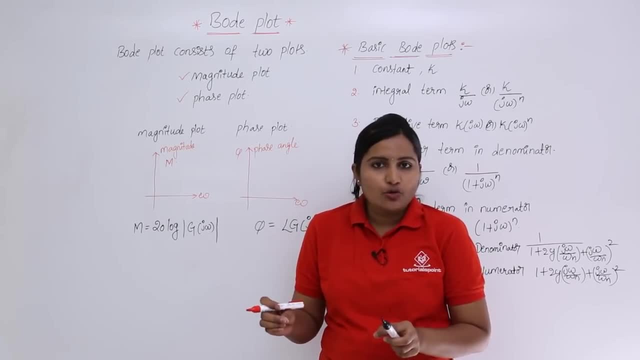 to consider as x axis. that means with reference to omega. we need to plot the magnitude by changing omega. we need to calculate for different values of omega. we need to calculate this value and by plotting this value with respect to omega, you are going to get your magnitude plot. 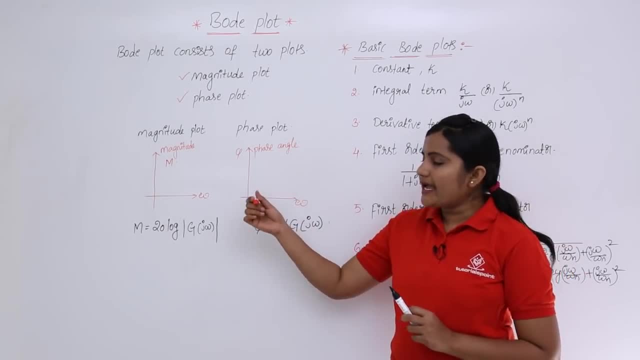 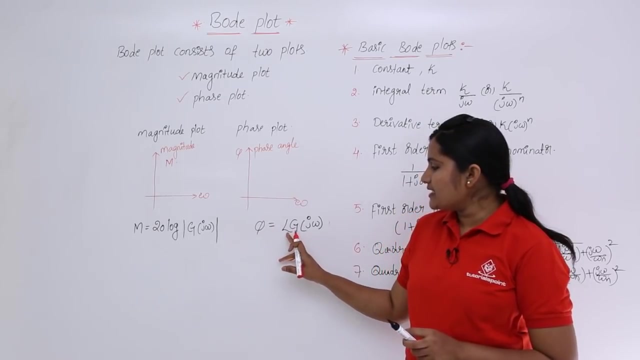 Coming to phase plot. so, as I told you, y axis is different for both magnitude and phase plot. for phase plot the y axis is equivalent to phase angle, phase angle of open loop transfer function. So here phi is equivalent to angle of open loop transfer function. means g of j, omega, here also. 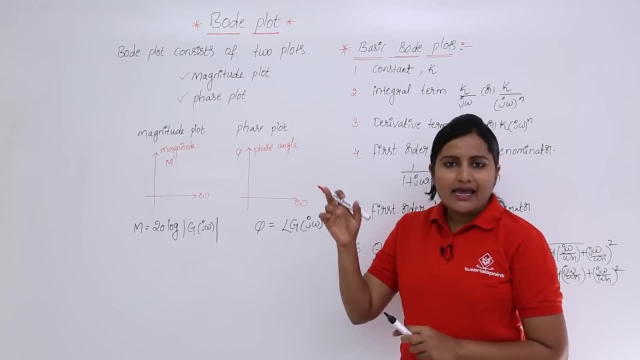 phi is equivalent to general equation will be angle of g of j omega into h of j omega. as our ideal system is unity feedback system, I am going to consider without h of j omega. that means phi is equivalent to angle of g of j omega. Now, 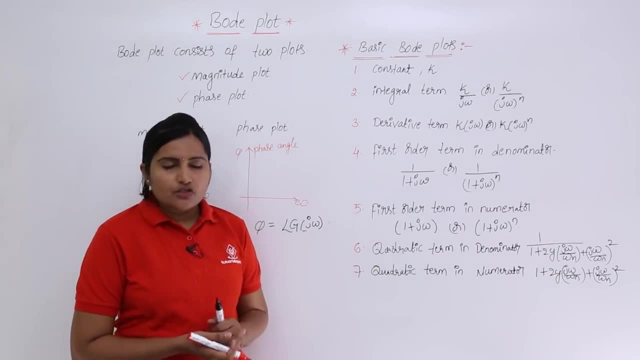 what testing will we have coming to different basic bode plots? So definitely you are asked to find out the bode plot or the analysis from bode plot for this reference structure, Only from these basic structures you are going to ask, you will get questions. so that means, for example, if you 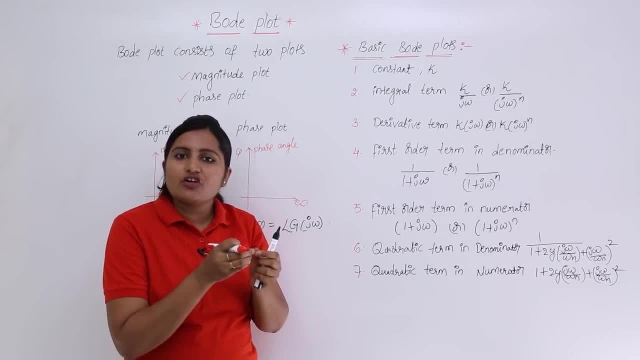 are having for constant K. if you know the constant K bode plot, The system is basically working approximately bode plot. you can trace bode plot for any constant. that means k or 2 k or 3 k or 4 k. the bode plot will be similar. So that is why we are having so many basic bode plots. 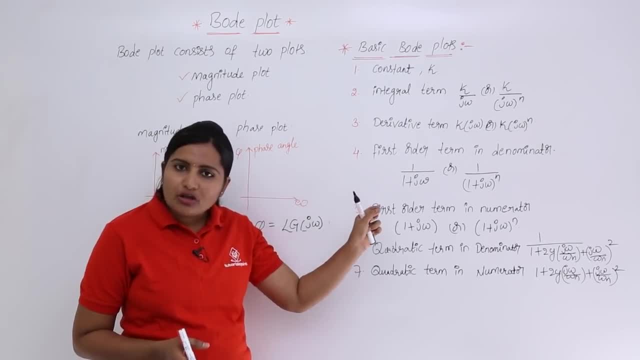 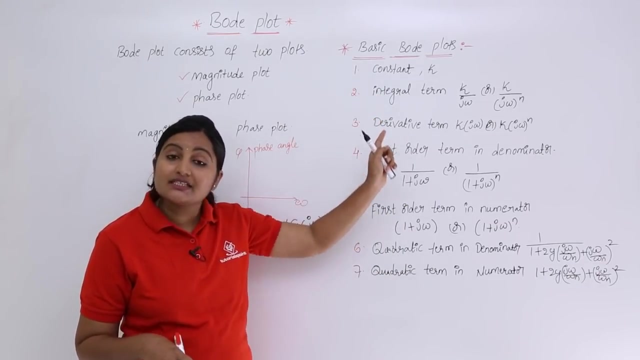 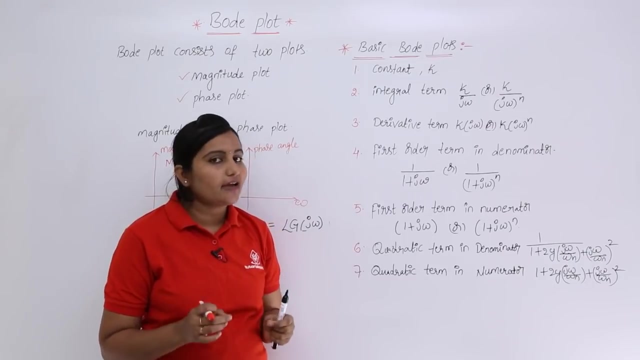 like this: If you draw that bode plot for this basic structures, you can easily analyze the bode plots for those which are having this reference, which has, which are having this forms. So now here, the basic bode plots are constant k for constant k. we are going. 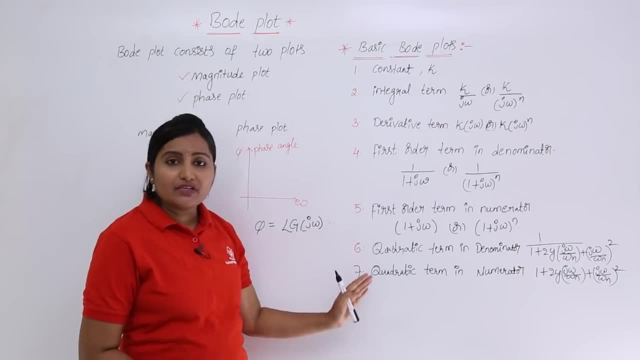 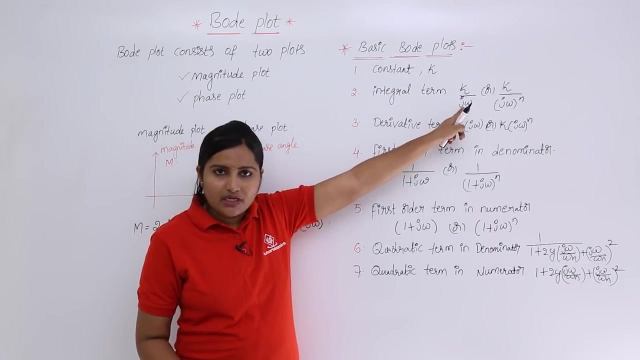 to draw bode plot. from the next class onwards we are having 7 different videos. we are having different videos to draw main bode plots in this list, So integral term. So next we are going to draw integral term, Bode plot for integral term. integral term is k by j omega or k by j omega, whole power. 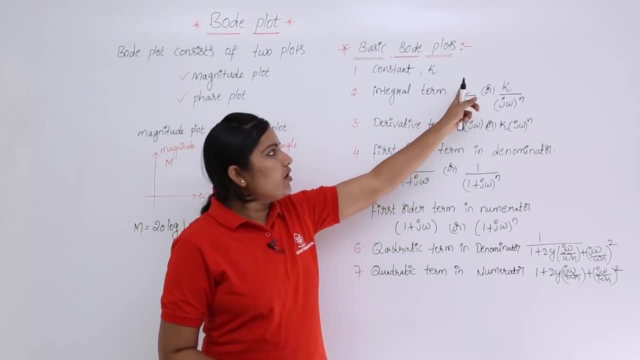 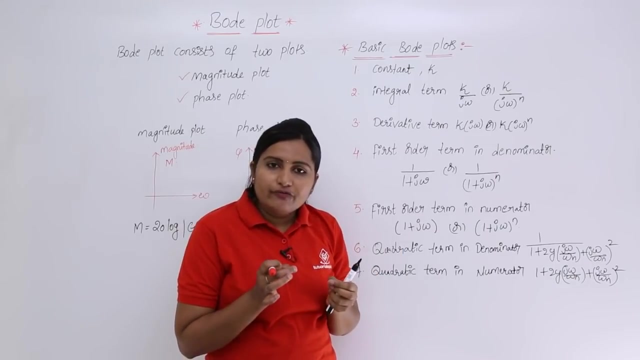 n. So integral term always will be in ratio, always will be in denominator. You can see: integral term is 1 by j omega, 1 by j omega whole power n, or k by j omega or k by j omega whole power n. If you completed this bode plot, you can trace the bode plot for 1 by: 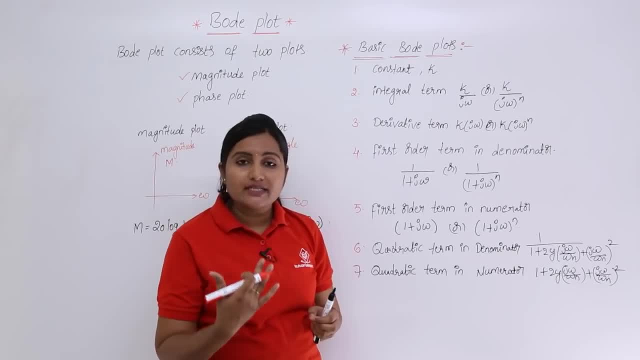 j omega. 1 by j omega whole power n. 2 by j omega, 2 by j omega whole power n. 3 by j omega, 3 by j omega whole power n. so on n by j omega and n by j omega whole power n. 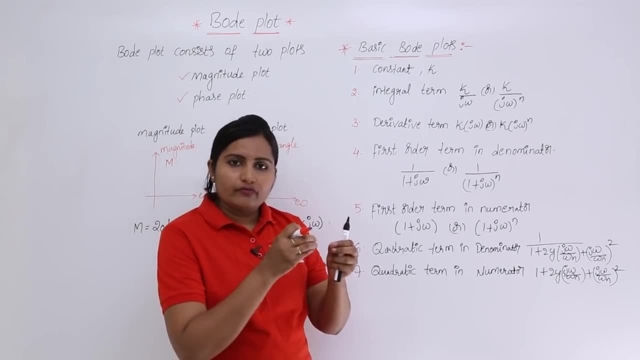 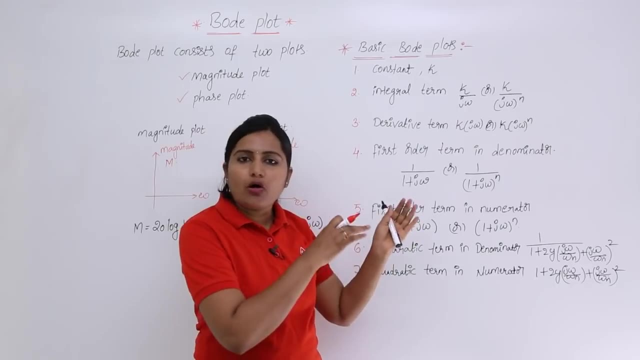 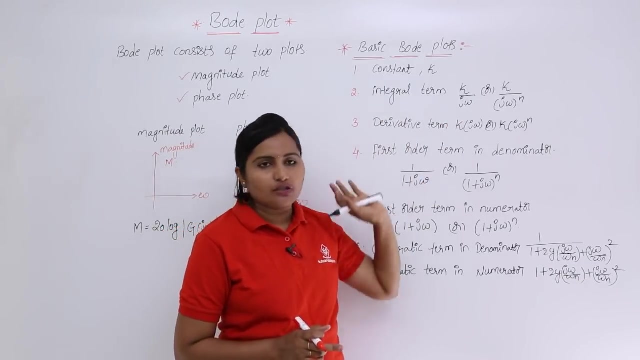 So that means whatever values, whatever the terms which are in this form we can trace bode plot for all those terms if you know bode plot for this. So similarly derivative term. So whenever you had a derivative term, there will not be any ratio here. So k into: 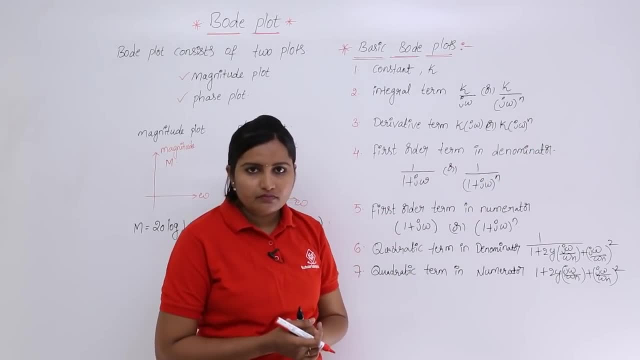 j omega k into j omega whole power n. This is derivative term Coming to first order term in denominator. First order term means 1 by 1 plus j omega or 1 by 1 plus j omega whole power n. Here the order is 1.. So first order term in denominator. Denominator means 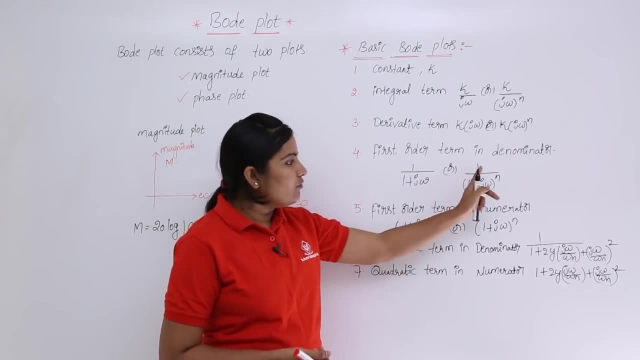 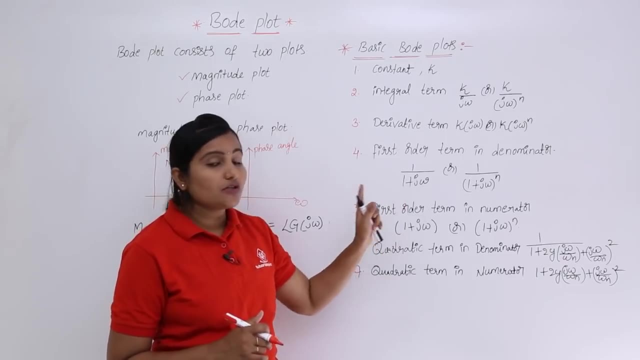 so we are having ratio 1 by 1 plus j omega, 1 by 1 plus j omega whole power n. This is one of the example for first order term in denominator. For this also we are going to draw the bode plot And coming. 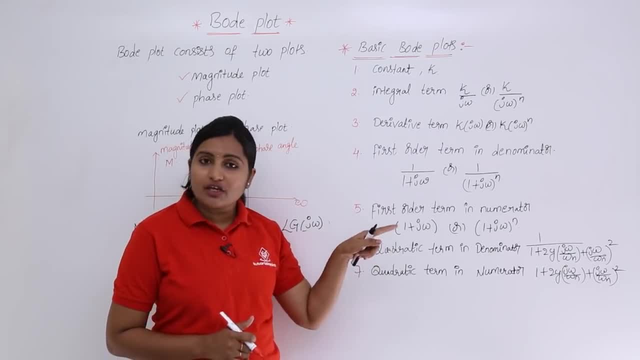 to first order term in numerator. So for this also we are going to draw the bode plot. So that means 1 plus j omega or 1 plus j omega whole power n. So for this, if you completed bode plot then you can trace k plus j omega, k plus j omega whole power n. 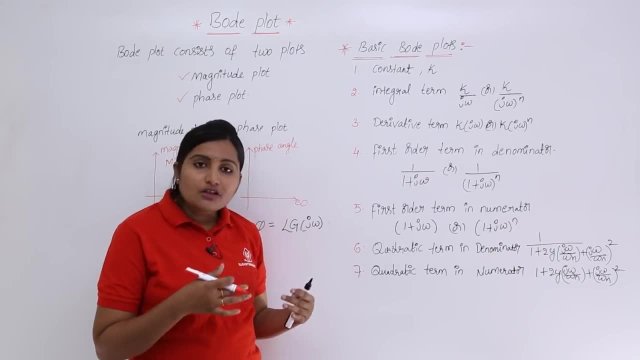 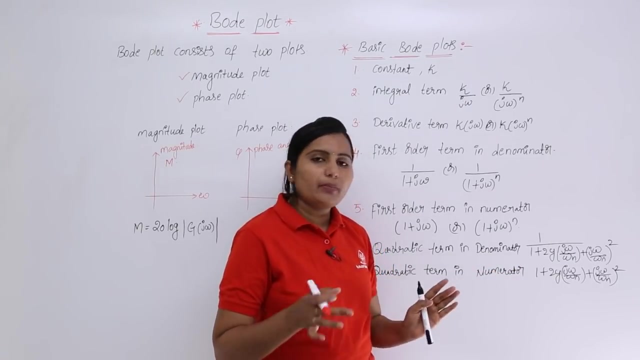 2 plus j omega For all this. you can do the same procedure Now. quadratic term in denominator. So this is the quadratic term in denominator For this type of terms. if you completed bode plot, you can apply for this type of terms. That means so here: quadratic term in denominator. 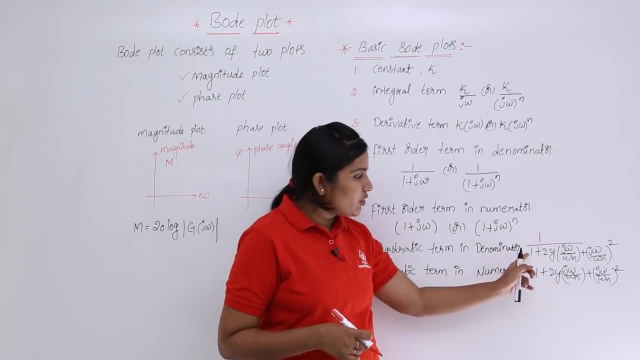 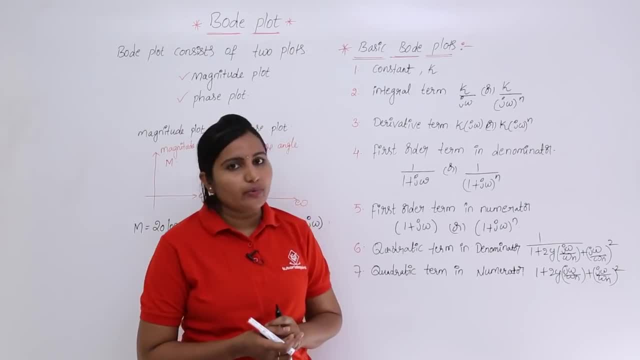